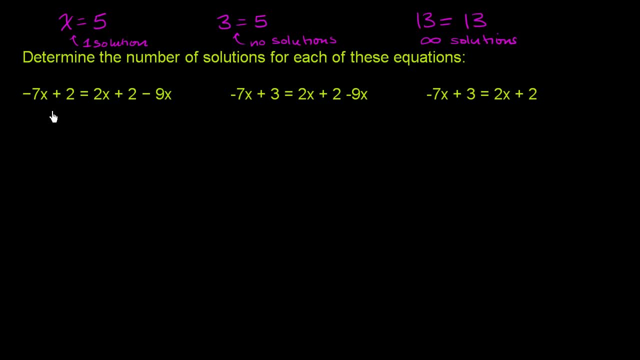 let's try to tackle these three equations. So over here let's see, Maybe we could subtract- if we want to get rid of this 2 here on the left-hand side, we could subtract 2 from both sides. If we subtract 2 from both sides, 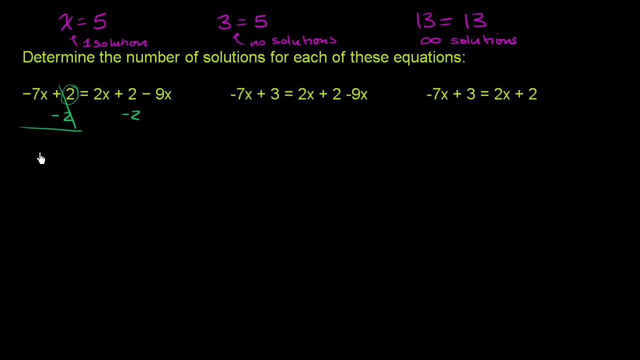 we are going to be left with. on the left-hand side, we're going to be left with negative 7x, And on the right-hand side, you're going to be left with 2x. This is going to cancel minus 9x. 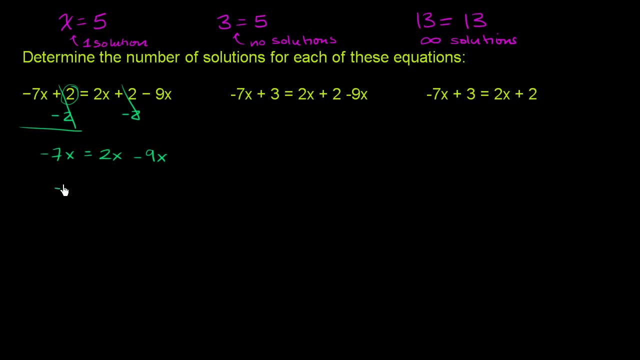 2x minus 9x. if we simplify that, that's negative 7x. You get negative 7x is equal to negative 7x And you probably see where this is going. This is already true for any x that you pick. 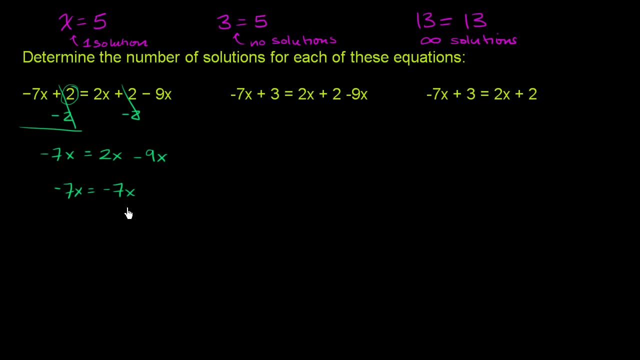 Negative 7 times that x is going to be equal to negative 7 times that x. So we already are going into this scenario. But you're like, hey, so I don't see 13 equals 13.. Well, what if you did something like you divide both sides. 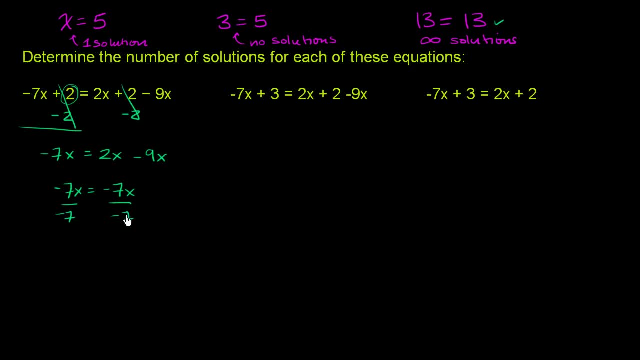 by negative 7?. At this point what I'm doing is kind of unnecessary. You already understand that negative 7 times some number is always going to be negative 7 times that number. But if we were to do this we would get: x is equal to. 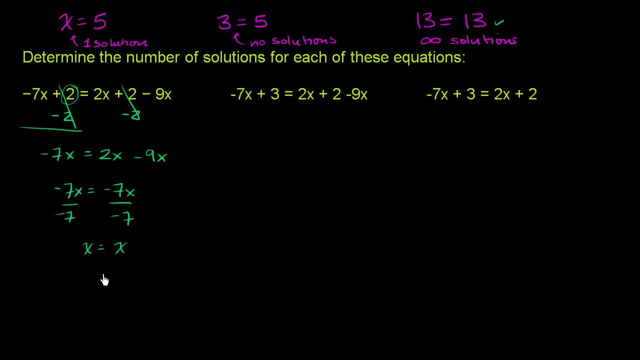 equal 2x, And then we could subtract x from both sides, And then you would get 0 equals 0, which is true for any x that you pick. 0 is always going to be equal to 0. So any of these statements are going to be true for any x you. 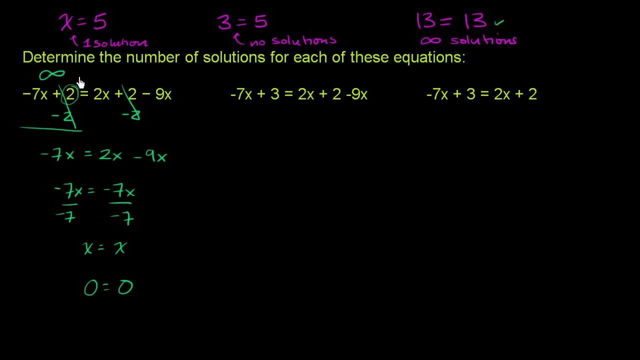 pick. So for this equation right over here, we have an infinite number of solutions. Let's think about this one right over here in the middle. So once again, I'll do it a little bit different. I'll add this: 2x. 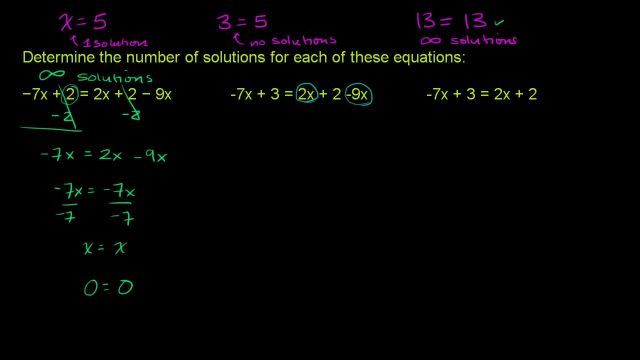 And this negative 9x right over there, So we will get negative 7x plus 3 is equal to negative 7x. So 2x plus 9x is negative 7x plus 2.. Well, let's add. 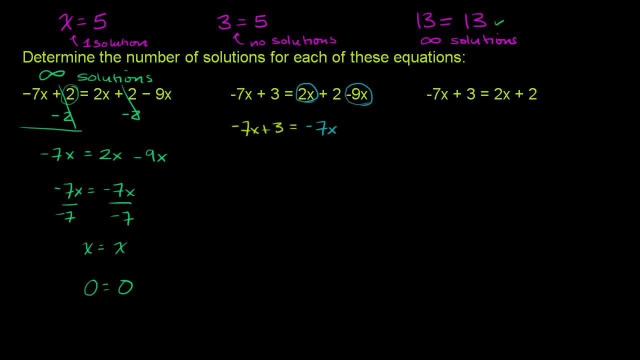 Actually, we'll do that in that green color. Let's do that in that green color Plus 2.. That's this. 2. Now let's add 7x to both sides. Well, if you add 7x to the left-hand side,